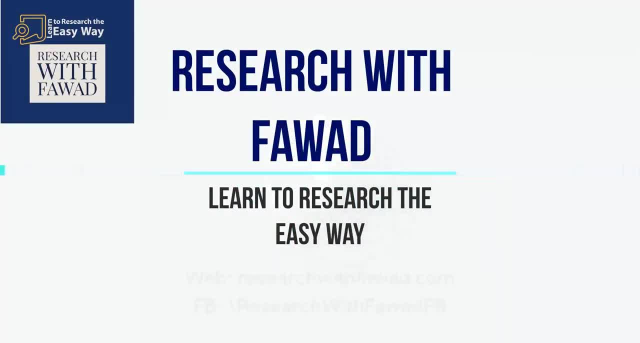 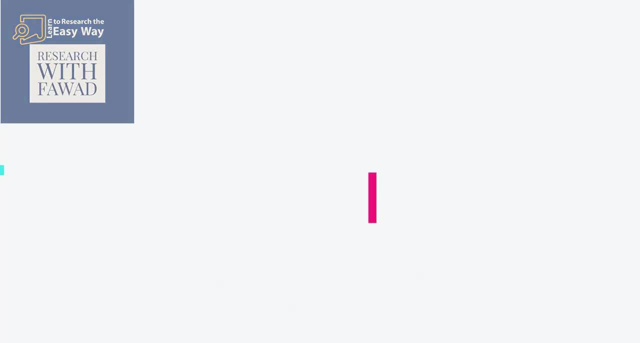 Outliers. In this session, we are going to talk about outliers. At the end of this session, you should be able to understand how to identify outliers and how to identify the level of z-score for a response that typically indicates an outlier Outliers: One of the major concerns when analyzing data is the effect of outliers, which are unusually. 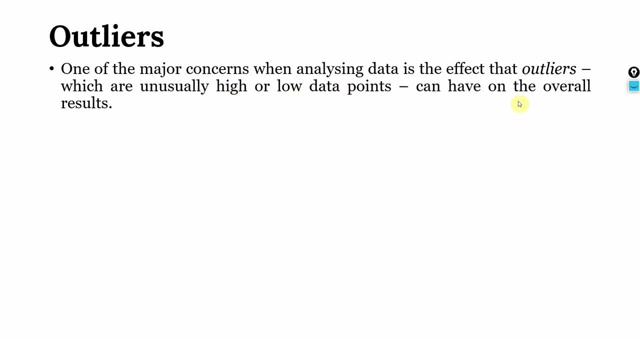 high or low data points, and they can have an impact on the overall results as well. For example, if you were asking everyday people how many cups of coffee they consume a day and most of the responses were between zero to four, that would be a normal spread of. 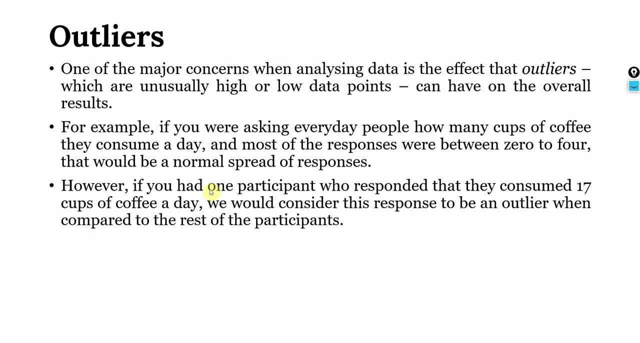 responses. However, if you had one participant who responded that they consumed 17 cups of coffee a day, we would consider this particular response as an outlier when compared to the rest of responses that were between zero to four. This is considerably away from the standard. 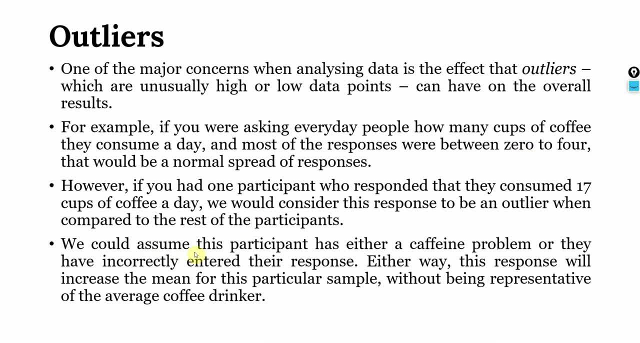 response. Now we could assume this participant has either a caffeine problem or they have incorrectly entered their response. Either way, this response will increase the mean for the particular sample without being representative of the average coffee drinker. Now, once you add this 17 with existing data, this is going to increase the mean manifold. 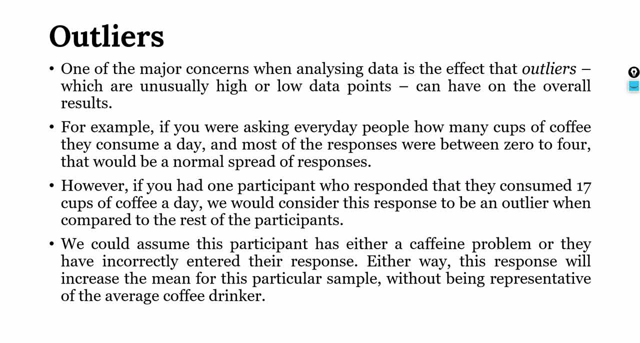 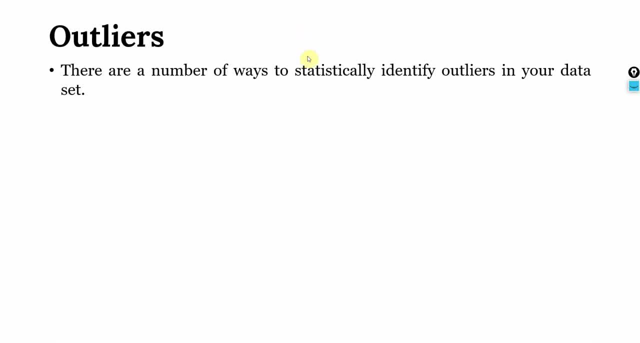 and which will not be a true depiction of the responses of the majority of the respondents. Now there are a number of ways that you can use to assess the outliers statistically. Now check for descriptive statistics, check for minimum and maximum values. Now we are going to look into each of these ways in SPSS. 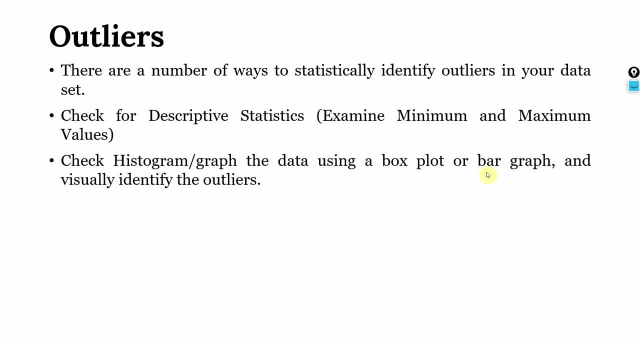 Now check for histogram graph the data using a boxplot or bar graph and visually identify the outliers. Now we can see that the participants responses to any variable can be transformed to a z-score, which is the basic transformation, allowing you to compare responses across cases to a. 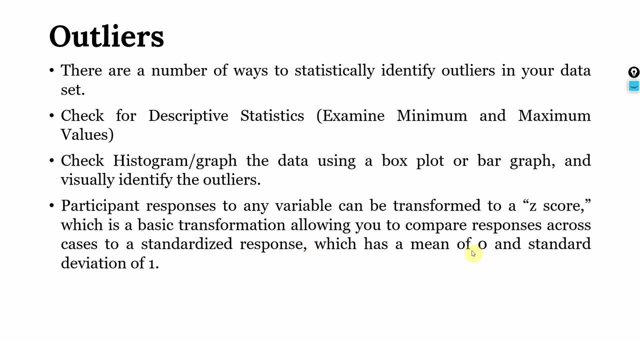 standardized response which has a mean of zero and a standard deviation of one. So what you can do is you can transform the participants responses to a z-score and that can obviously highlight the outliers as well, And if your z-score is greater than 3.3 plus, 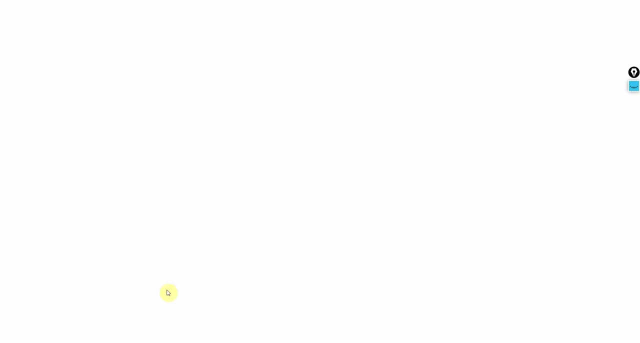 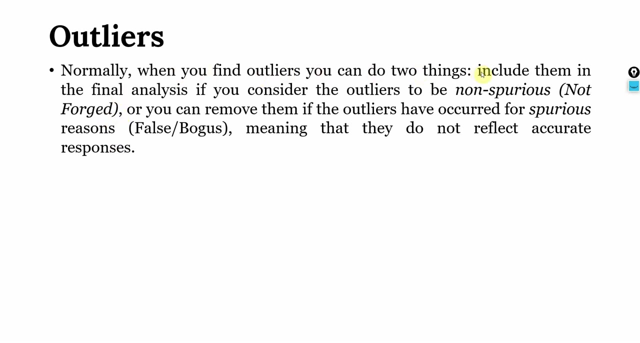 or minus, it can be considered as an outlier. Now, normally, if you find outliers, you can do two things: include them in your final analysis if you consider them not forged or non-spurious, or you can remove them if the outliers have occurred for false or bogus reasons. 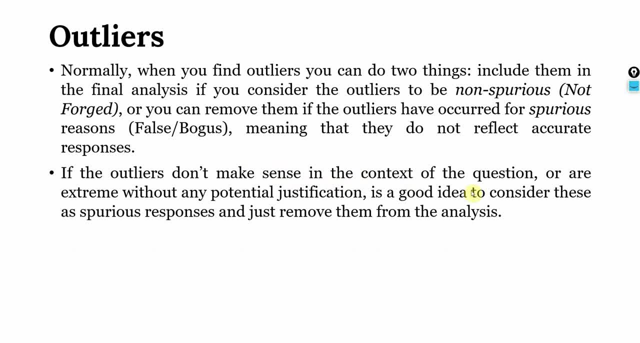 Now, if the outliers don't make sense in the context of the question or are extreme without any potential justification, it's always a good idea to find them Now. if the outliers don't make sense in the context of the question or are extreme without any potential justification, it's always a good idea to find them. 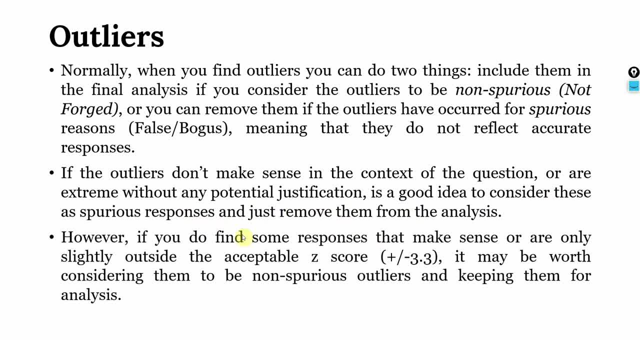 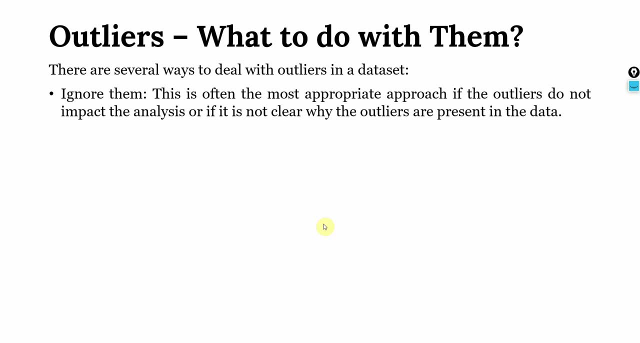 that these responses shall be removed. however, if find the responses that make sense and are only slightly over the Z score of 3.3, then you can keep them. now again, what to do with them? now there are several options. you can ignore them if they are not affecting your responses or your data a great deal. you can trim them. 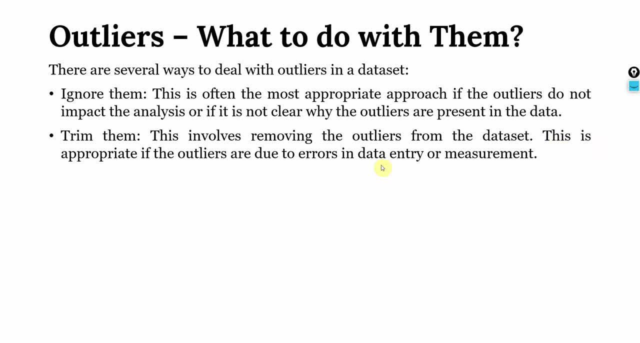 this involves removing the outliers from the data set, and this is appropriate if the outliers are due to errors in the data entry measurement. now for this: if you are doing survey based analysis, a good idea is go back to the field questionnaire in hard form or maybe, if you have imported them- maybe you have. 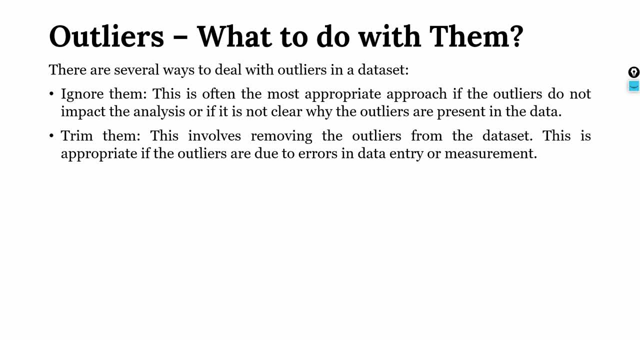 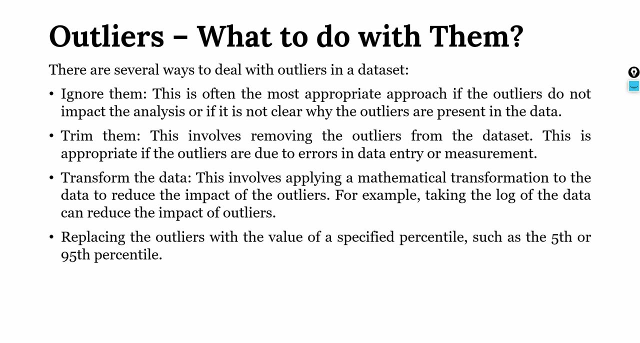 made a mistake while doing something. just double check your original data now, transform the data, and this is by taking the log of the data and it can reduce the impact of outliers. so you can do mathematical transformation you now. otherwise you can do replacement of the outliers by identifying the fifth. 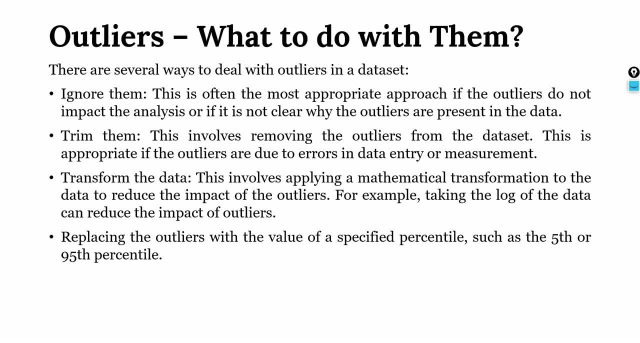 and ninth percentile score. so if there is an outlier, replace it with a fifth or 95th or 95th percentile score. now it is very important to carefully consider the appropriateness of each approach, as removing or ignoring outliers can sometimes distort the analysis and lead to incorrect conclusion. now what we are. 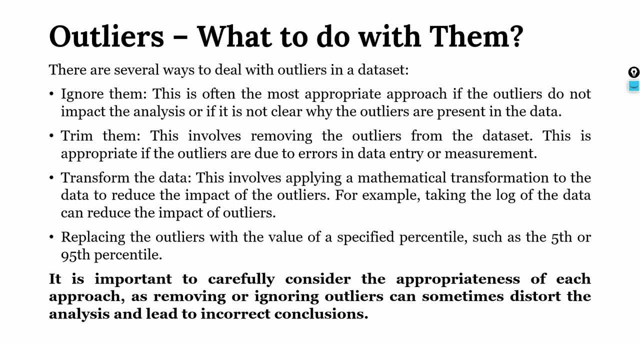 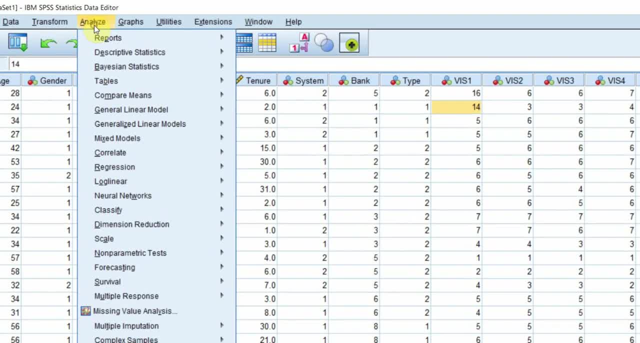 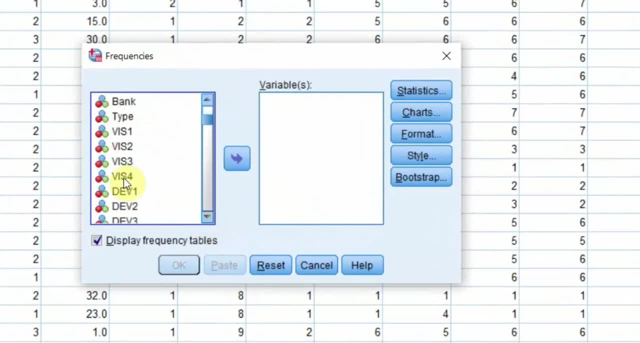 going to do is we are going to identify the outliers using SPSS now. now we are going to assess outliers in SPSS now. the first, easiest way is go to analyze descriptive statistics. let's go to frequencies and let's say: I am interested in this particular variable, region 1, so select it, edit here. go to statistics, select. 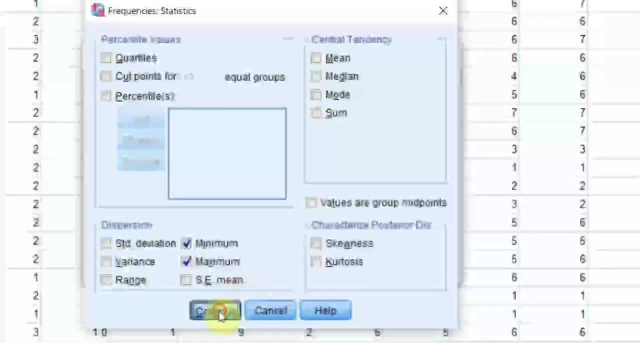 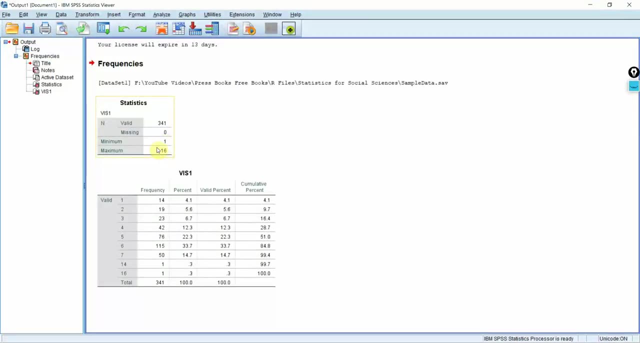 minimum, maximum press, continue, press, ok. and here, if you look here, minimum is 1, maximum is 16. now this is an outlier. now there are outliers here because the values are going beyond the maximum limit, which is 7. so look at this: there is a number 14. 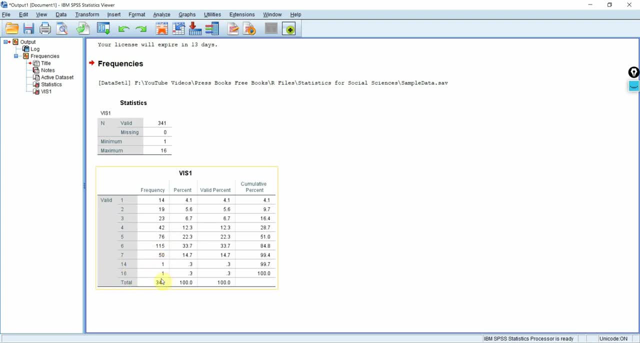 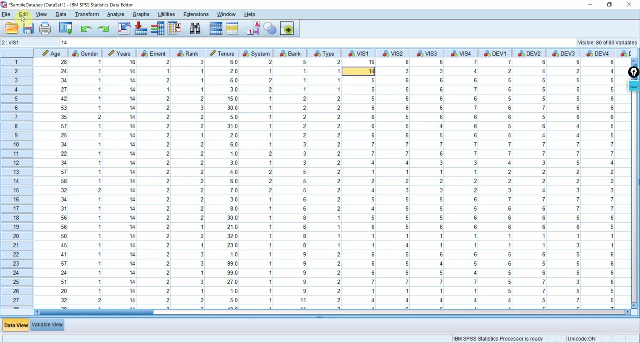 in here. the frequency is 1, number 16 and the frequency is 1, so it shows that there are two observations that actually are not within the range. so how do you find those observations? just go to Edit, find. and let's say, the first one was, if I'm not wrong, 14 and it was in Vision 1. 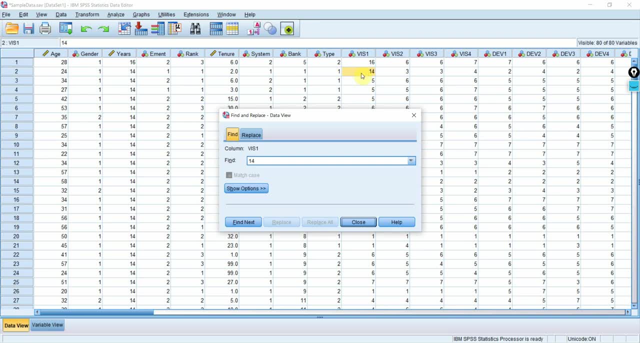 selected find next and it will give you that particular cell highlighted. now, here it is. it is case number two, so you can go to your original data set. or, if you've got collected, or if you've got data in hard form, just go to the response number two and see. 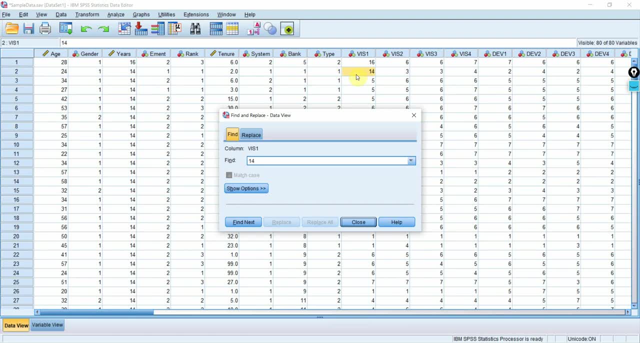 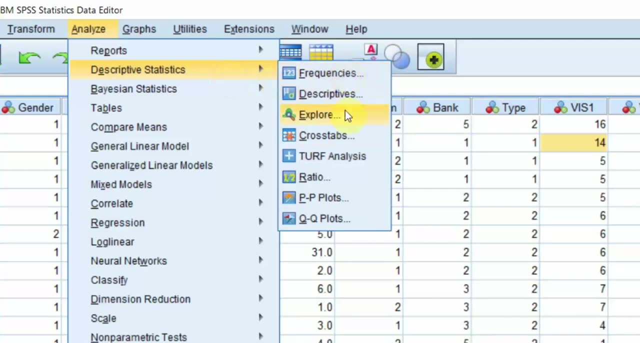 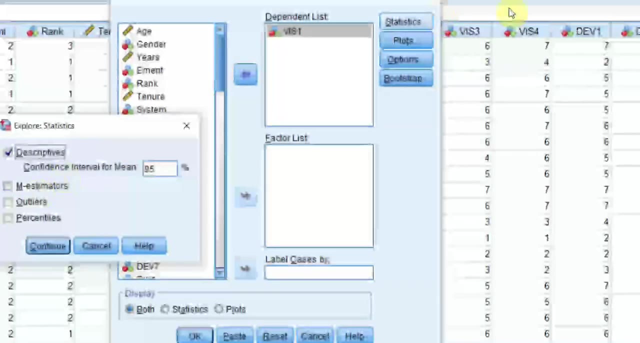 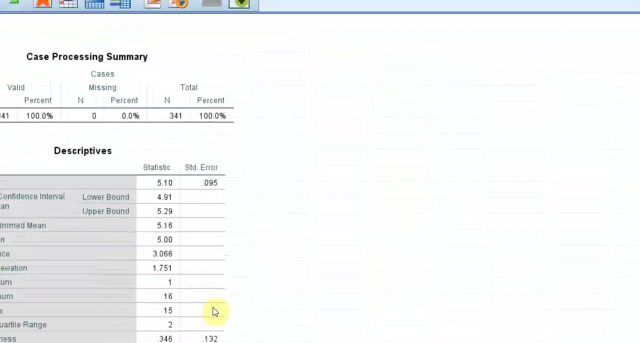 what the value was, and you can simply change it here now. the other way is go to analyze descriptive statistics, explore, let's say, vision one, and now i'm going to use statistics, outliers, press, continue and simply press. ok, now we are going to use box plot. so if you look here, there, 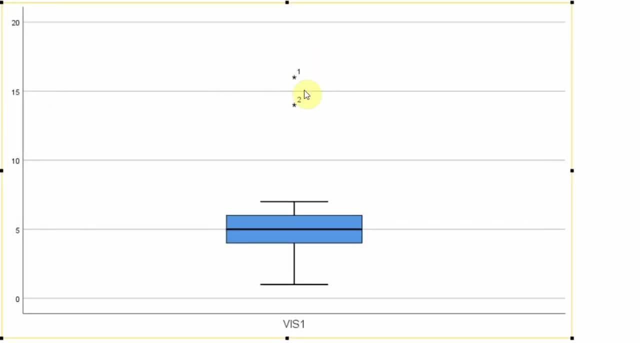 is a star here and there are the two, observation one and two. now they are far away from the range- the lower range and the upper range- and there is a star next to them. this means these are extreme outliers number one and observation number two. now again, you can go back to them.